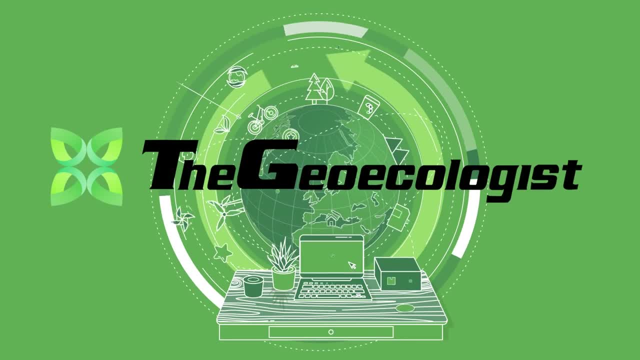 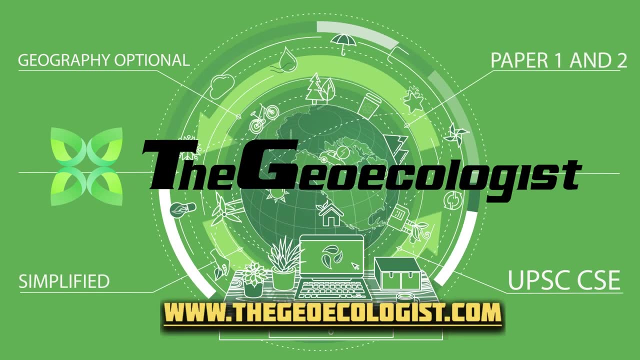 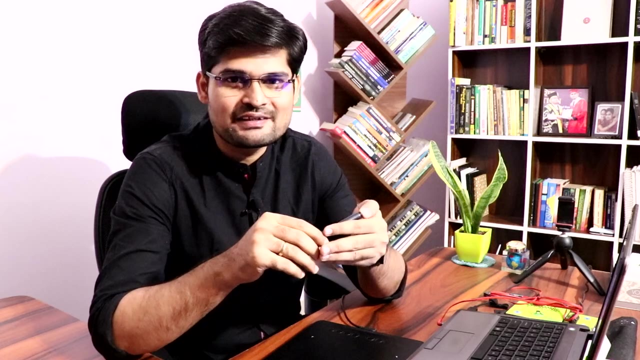 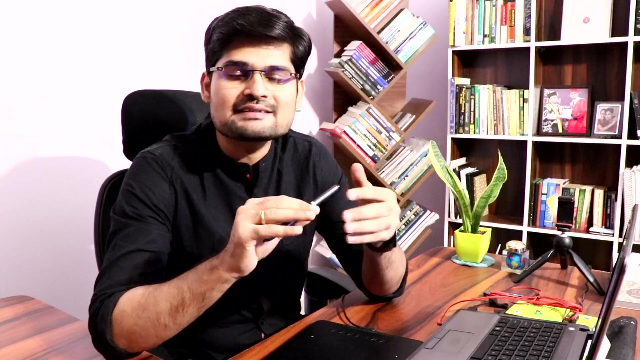 Hello everyone, welcome to the Geoecologist. I am Dr Krishnanand and you have been watching my videos on geography and various topics of geography. So in this session on biogeography, we are going to learn about the various aspects of soil formation, the factors of soil formation. 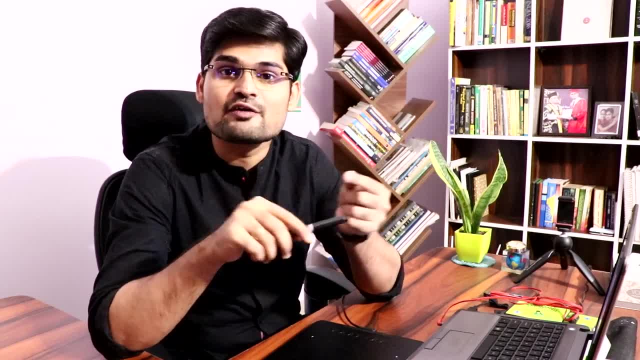 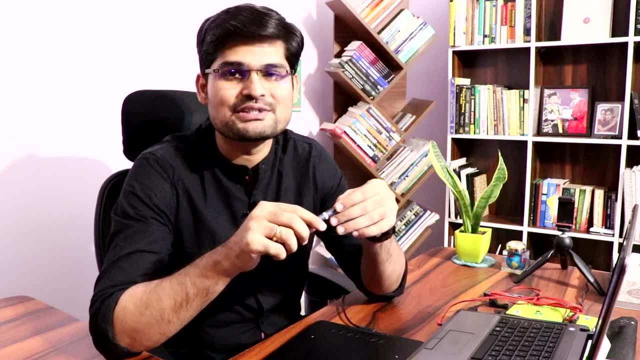 the processes when those factors undergo for the formation of soil across the world. So we are going to learn in details, But before we go ahead, please don't forget to subscribe to our channel and also do share the videos with others as well. So now let's learn about. 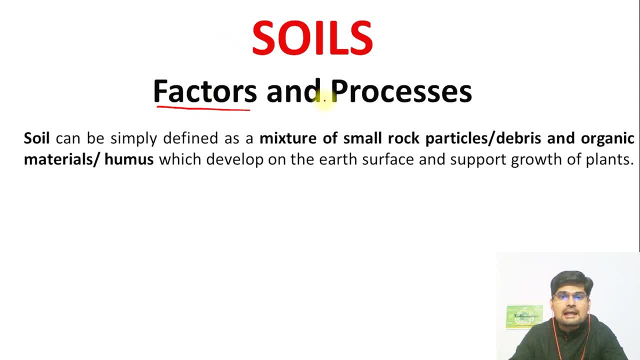 the soils, its various factors of formation and the processes of formation in this particular lecture. So there is a difference between factors forming soil and when those factors go under different processes. So we are going to learn about various factors and the processes that are important for the soil formation. But before we go ahead, the first important 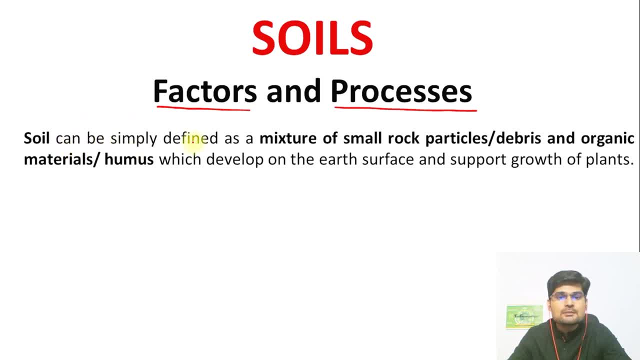 point is to define the soil formation. So soil can be simply defined as a mixture of small rock particles or debris particles. That is important to remember here that it's not an element or a compound. rather it is a mixture and it is made up of small rock. 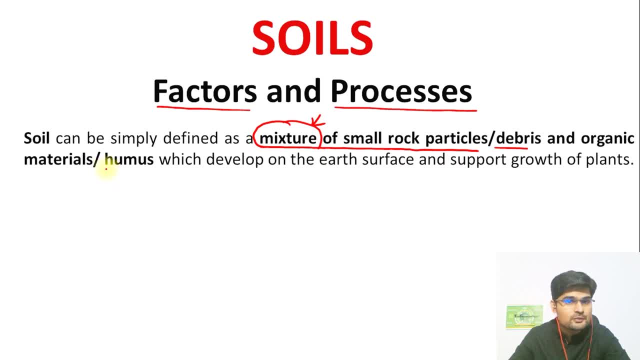 particles, debris particles and organic matters like humus, sand, sandstone, sandstone, sandstone, sandstone. So when you look at soil formation, it is a creative process which develops on the earth's surface and supports the growth of plants. That's the simplest definition. 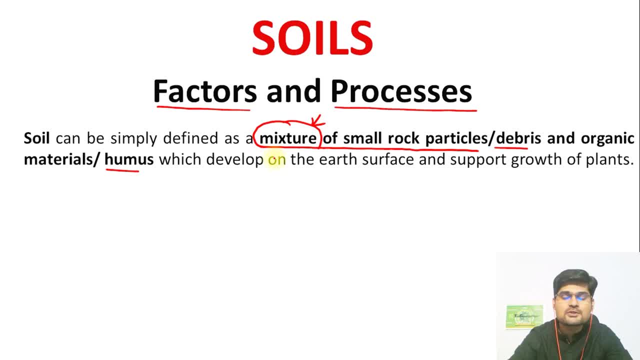 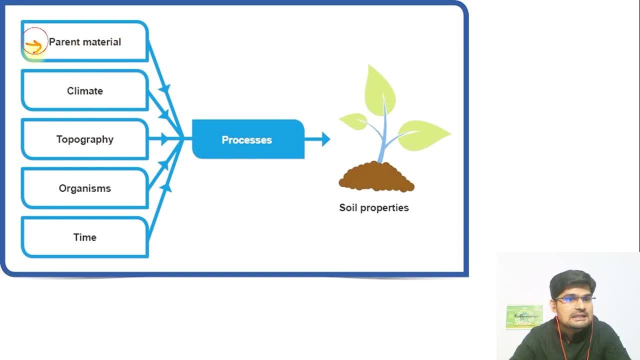 of soil. Now let's go to the factors of formation of soil. So what are the various factors? If you look into this flow diagram, you can see the first factor is the parent material right. So for genesis of soil the parent is important. And when we say parent material, 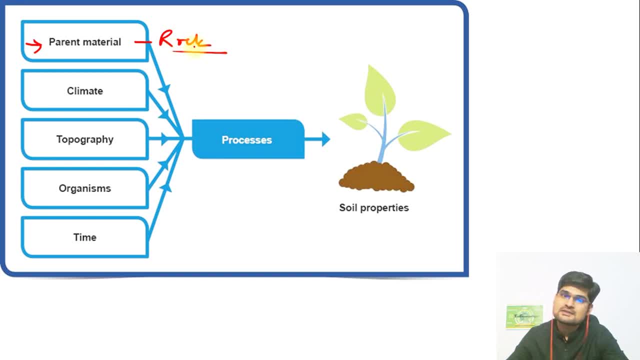 it is signifying the rock types, remember sedimentary rock, igneous rock, metamorphic rock, parent material for the soil formation. then we have the second factor, that is the climate. then what we have is the third factor, which is topography, and then we have fourth factor, which is organisms. that is where the organic 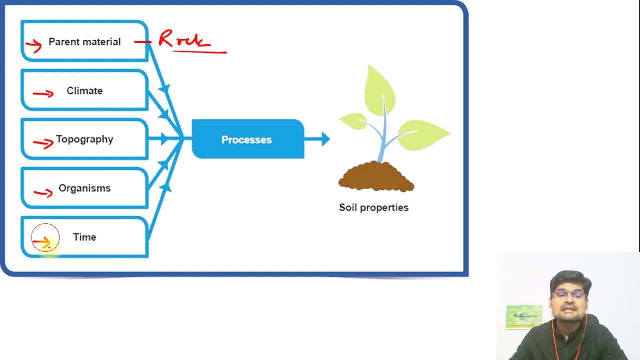 component comes to the soil, and the fifth and last component is time, which is most important of all, because soil does not form in a day. it takes lots of years, millions of years to form a layer of soil, and that is important. so what you observe here in this flow diagram are all these five factors and these 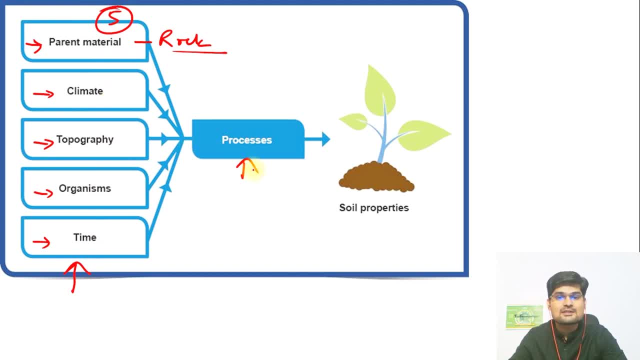 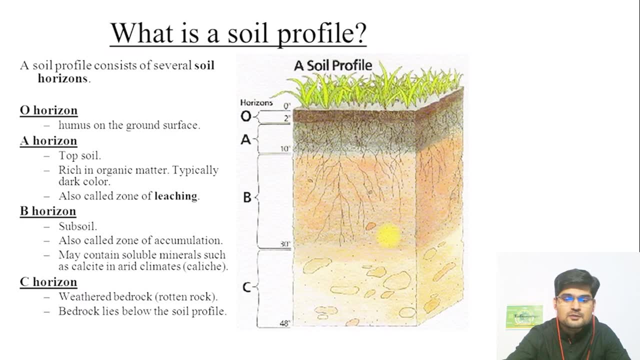 five factors go under different processes to form various soils with their unique properties. so now let's go ahead and discuss further more. so before we go ahead, let's understand the soil profile first. so soil profile is basically a general profile of the soil, that is, general layering or 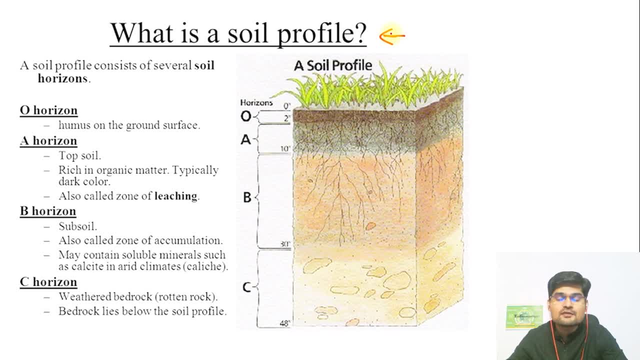 stratification of various components of soil. so when we say there are different layers of soil, then we are talking about different layers of soil that are formed under the soil after millions of years of evolution. so what is a general pattern? the general pattern is, alphabetically, O, A, B and C. so if you 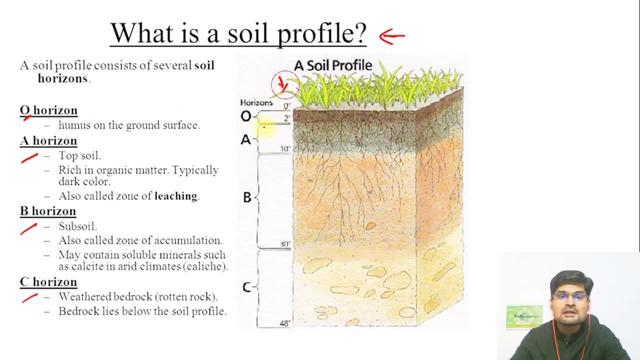 observe this: O, A, B, C, what you see here in this diagram. here that O layer is the topmost layer, which is from 0 to 2 feet- that is a general observation right- and which contains humus on the ground surface. that's important. and then you 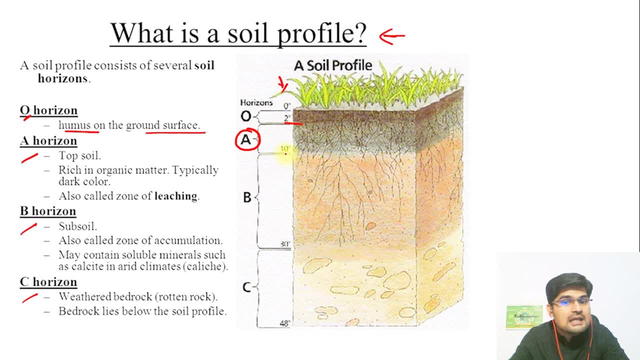 have horizon A now. a horizon ranges up to ten feet right and it is also called topsoil. so if you are confused, that O horizon is topsoil, remember horizon A is topsoil, not O. O is only containing the humus part right, the dead, decayed remains of plants and animals. and remember the. 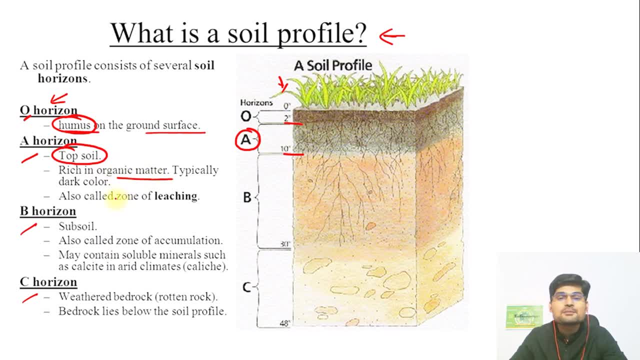 horizon A is also rich in organic matter and typically darker in color, as you can see here in the diagram as well. and remember this is also called zone of of leaching, and remember zone of leaching is where the soil loses the nutrient, So all the nutrient present in this layer is lost due to the various processes and it goes to the. 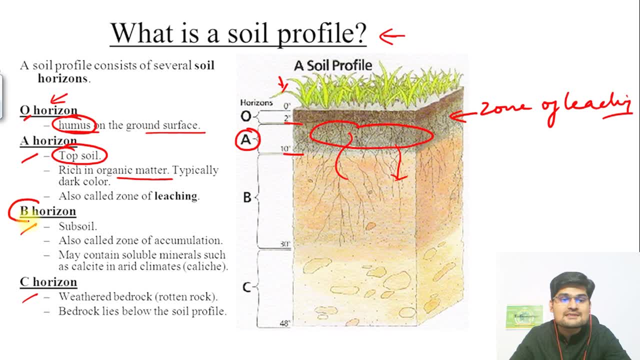 other layer and deposits further. So when you observe the horizon B after A, it is called subsoil because it is in subsequence with the soil. horizon A and also it is called zone of accumulation. Why? Because the above layer was zone of leaching from where in the next layer? 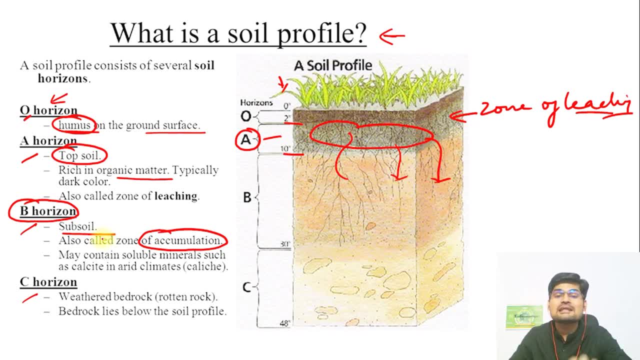 you find that all the nutrients go and percolate and finally accumulate, So that is why it is called zone of accumulation as well. It contains soluble minerals such as calcite in arid climates as well. and the sea horizon that is from 30 feet to about 48 feet. that is a general observation. 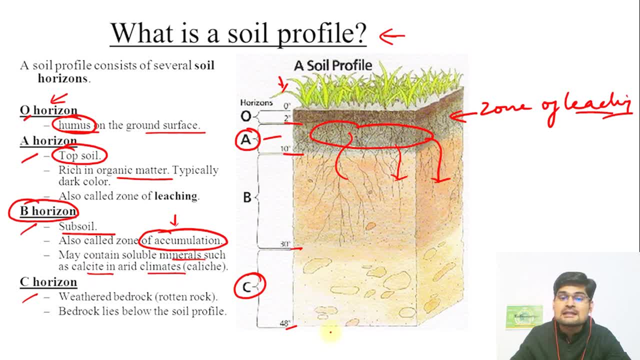 Remember, it contains withered rock materials and it is that layer that connects the entire horizon with the bed rock, and that is the most important point here. So this is a general observation of our soil profile. Now coming to the processes. So 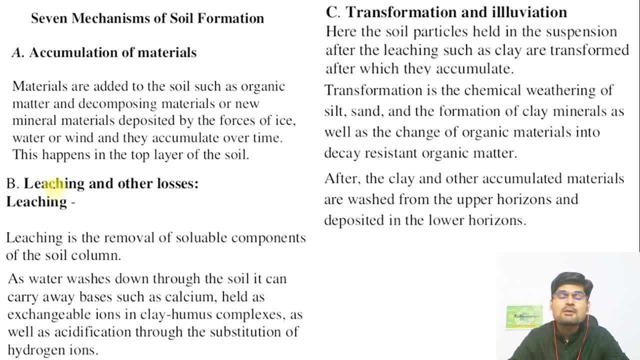 there are several processes that we need to discuss because, remember, soil formation is a very complex phenomenon and when, in biogeography, we try to decipher or decode the process of formation, there are several processes that we need to understand. So the first process is: 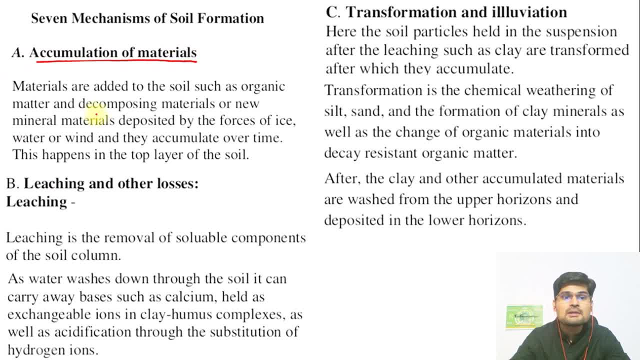 accumulation of the material. So the first process is accumulation of the material. So materials are added to the soil, such as organic matter and decomposing materials or new mineral materials deposited by different forces of ice, water, wind. They accumulate over time and 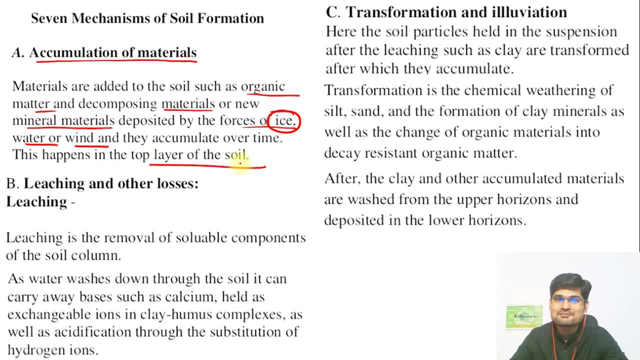 remember this happens where in the top layer of the soil. that is important. So the first process that we learn is accumulation. Then what we have is the leaching process. Remember leaching and losses that are important. So leaching is basically the removal of soluble compounds. 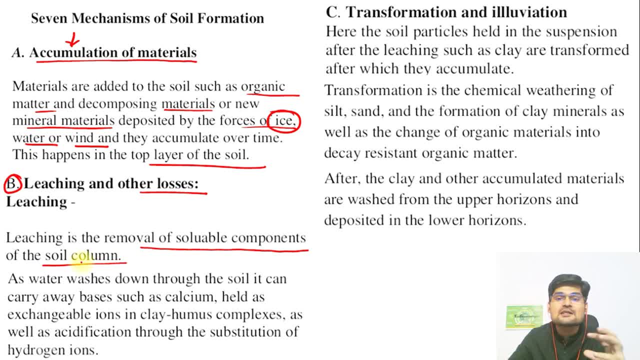 of the soil column. So when the soluble components are removed through the action of water- remember water washes down the soil nutrients and carries away the bases, such as calcium, held as exchangeable ions in the clay humus complexes and also as well as it is responsible. 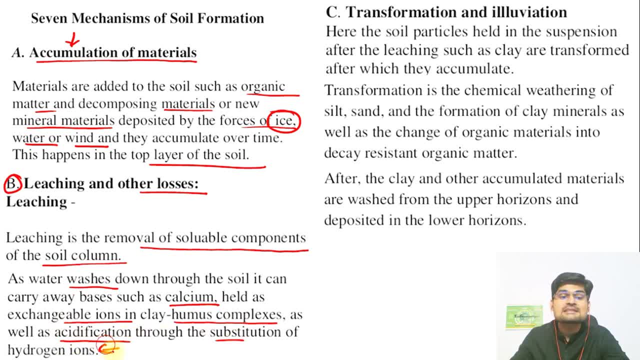 for acidification through the substitution of various ions as well many times. So leaching is another important process. So after that we have something called transformation and eluviation. Now, here the soil particles handled in the suspension after when they are leached, such as clay, are transformed, which they accumulate. So transformation is basically. 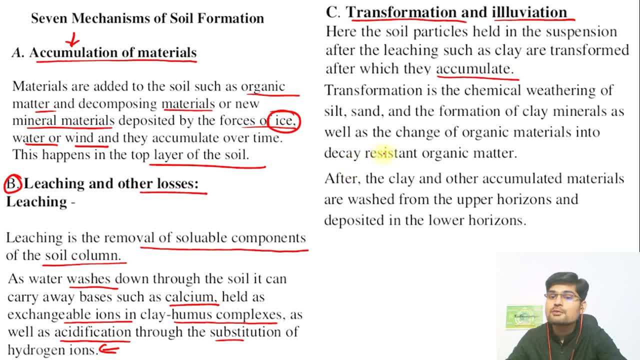 what? The change in structure, the change in chemical composition. So transformation is the chemical weathering of the silt sand and formation of clay minerals, as well as the change of organic materials into decay resistant organic matter. So that is important point to remember. and after that, 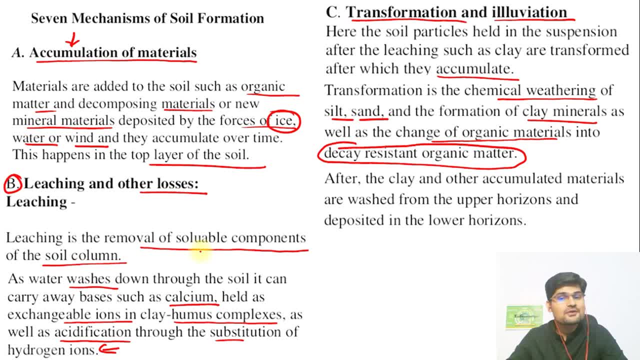 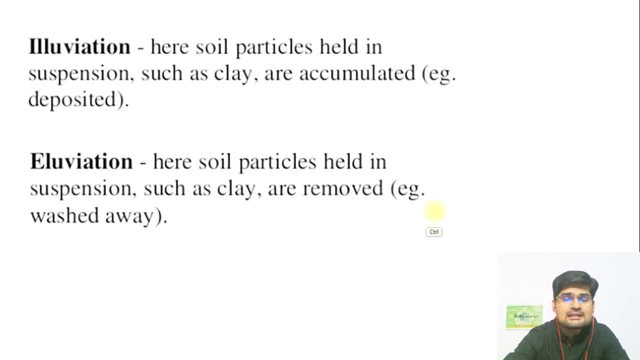 was bleed 요�, the other accumulated materials washed from the upper horizons and deposited into the lower horizons, as we saw in the last diagram. So that is important here. Now. there are 2 words that we must discuss here. One is called eluviation and the other is called elluviation, the word from. 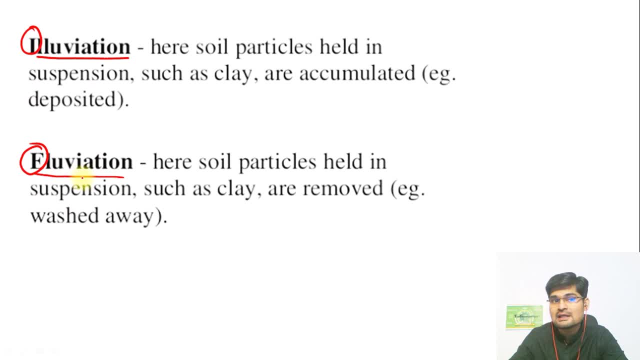 I and e. So what is the difference between these two? Remember, ellauviation Here refers to the soil particles held in suspension, such as clay, when they are accumulated, accumulated or deposited. So eluviation is the process of accumulation, right after when there. 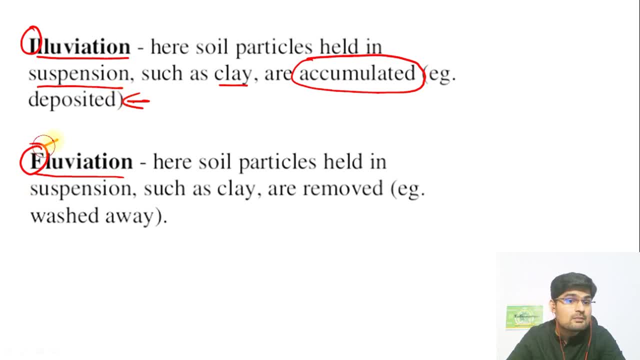 is leaching occurring, But eluviation, remember E here soil particles which are held in suspension, such as clay, are not deposited, rather they are removed or washed away. So when there is removal, remember it is eluviation from E right removal, while if it is deposition or accumulation. 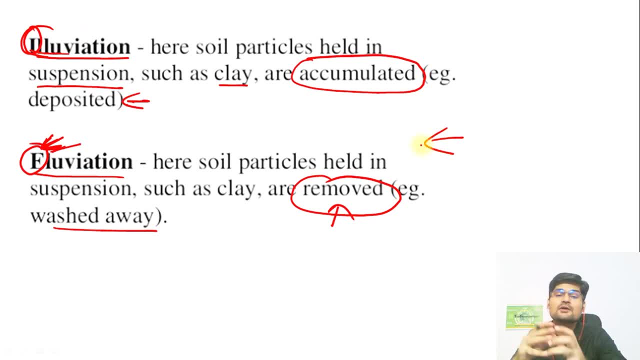 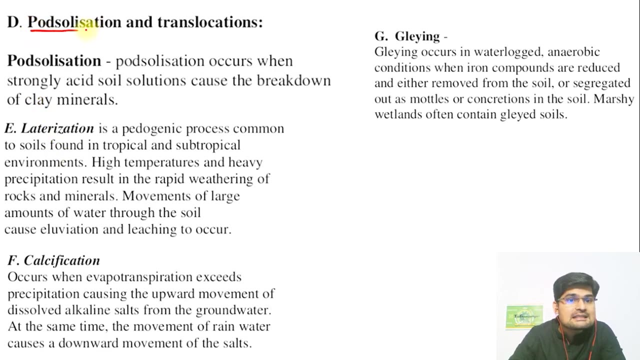 it is eluviation. So don't get confused while you are reading these words. Eluviation means deposition, eluviation, that is external, going away, wash away. So that is important point to remember here. Now let's go to the next process. This process is called podsolization, and 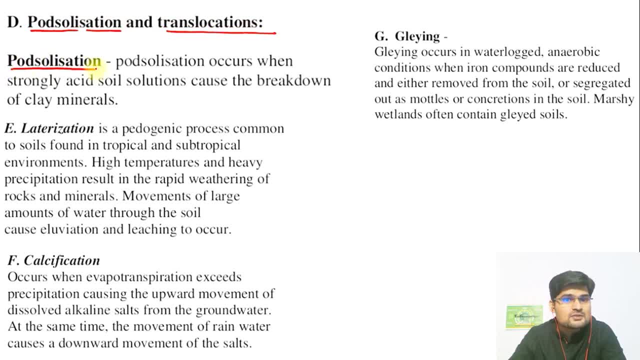 translocation. So what is this podsolization? So podsolization occurs when strongly acidic solutions of soil cause the breakdown of the minerals of clay. That is the most important point. So podsolization occurs when strongly acidic solutions of soil cause the 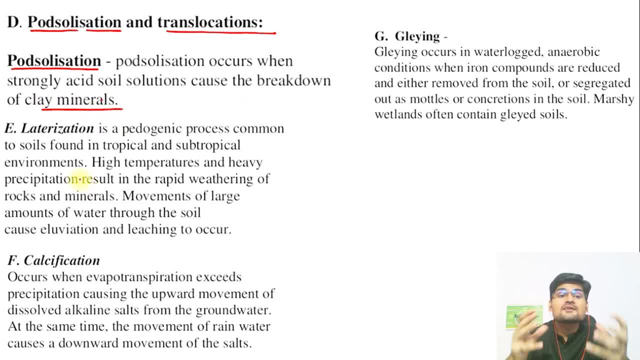 breakdown of the minerals of clay. That is the most important point. So it is like acid breaking the various clay minerals. right, that is called podsolization. And when we say podsolization there is also something called translocation. Now, remember, the word is trans, it means it is not. 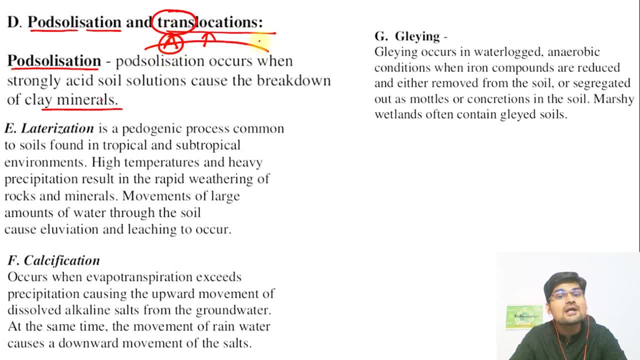 located at a particular place. rather, from one place it is going to the other place and getting translocated in the process while breaking down right. So that is important process. Now coming to the fifth one. it is called letterization. Now remember letterization. 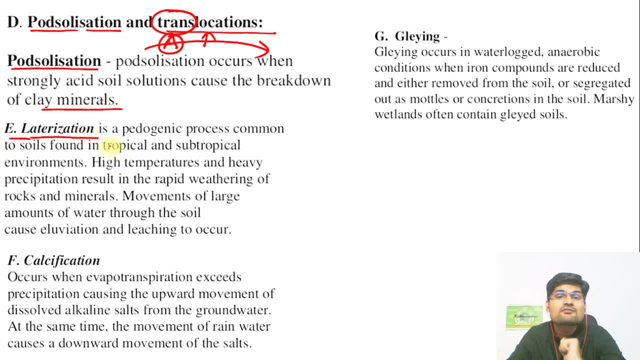 is important word here- as an important soil forming process, which is also called pedogenic process. And remember it is common where in the tropical and subtropical environment. Why? Because they have high temperatures and heavy precipitation. So where you have high temperatures, 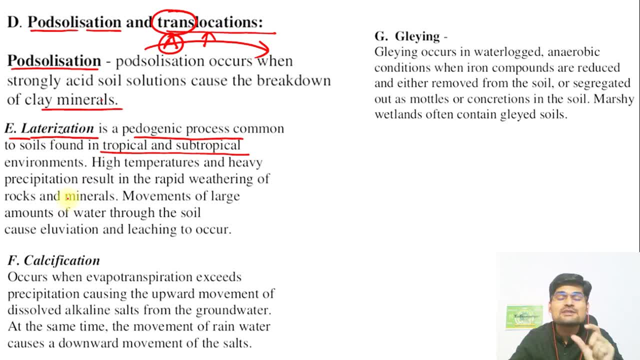 and heavy precipitation, what happens? There is a rapid withering of rocks and minerals. right, And also remember, movement of large amount of water through the soil leads to alleviation. That is basically the word for the process of pedogenic process. So when you have high temperatures and 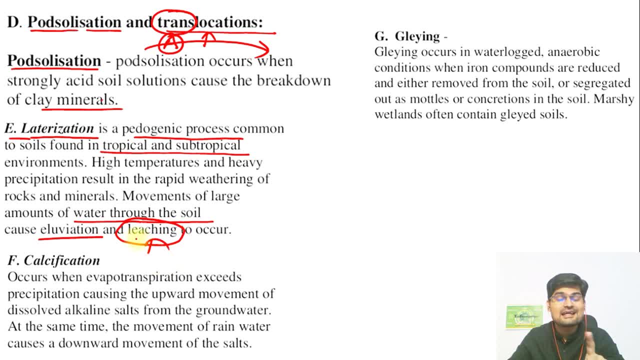 heavy precipitation. what happens? There is a rapid withering of rocks and minerals. That is basically going away, wash away, leaching, right, And that is where letterization process is important, right, Then what we have is something called calcification, As the name itself suggests. 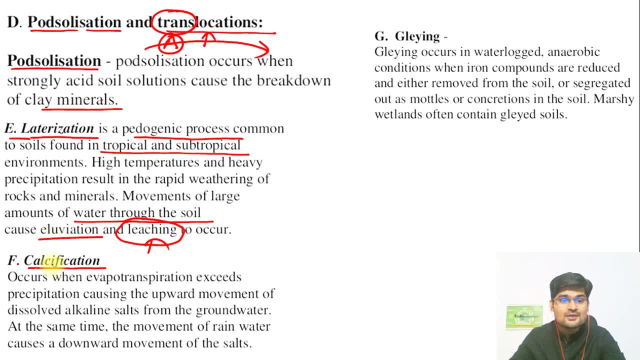 what is happening here? Calcium containing thing, right. So occurs when evapotranspiration exceeds precipitation. Remember, in areas where you have lots of temperature, right, high temperature. So what will happen? Evaporation is also high Transpiration through the nodes of the plant leaf. 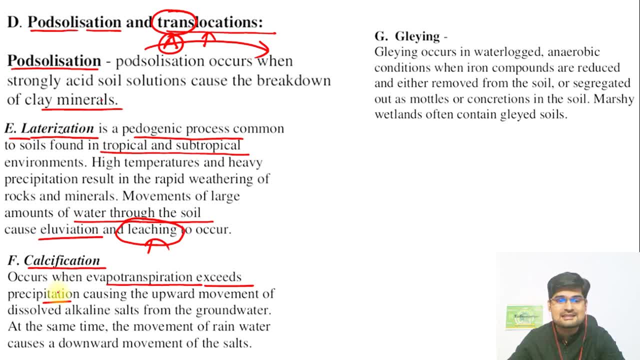 is also very high, But precipitation is less right. In such environment, there is upward movement of dissolved alkaline salts, like calcium salts, right from the groundwater, And this is where calcification occurs. So what happens? There is a deposition of calcium carbonate in the soil. 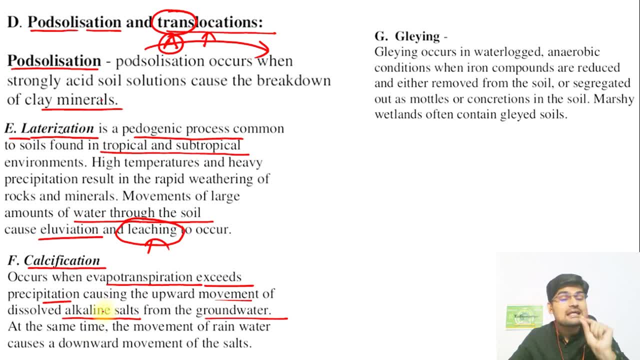 or so-called salt in the soil. That is where the alkalinity of the soil increases right. So at the same time, the movement of rainwater causes a downward movement of the salt as well in many parts of the world. So remember, calcification is important process of soil. 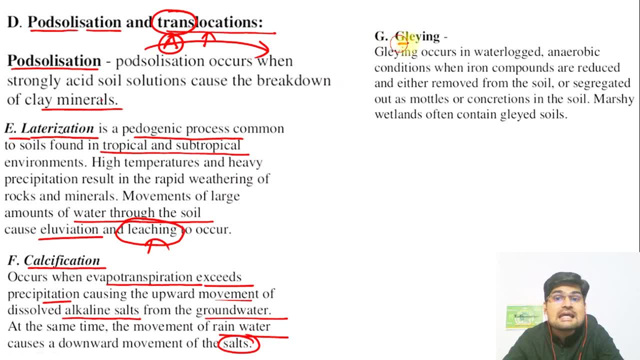 formation as well, Then what we have is something called glaying G-L-E-Y-I-N-G. So what is this glaying and where does it occur? Glaying occurs in waterlogged anaerobic conditions. when, remember, it is saying anaerobic condition, that is, lack of oxygen, right? So when it is? 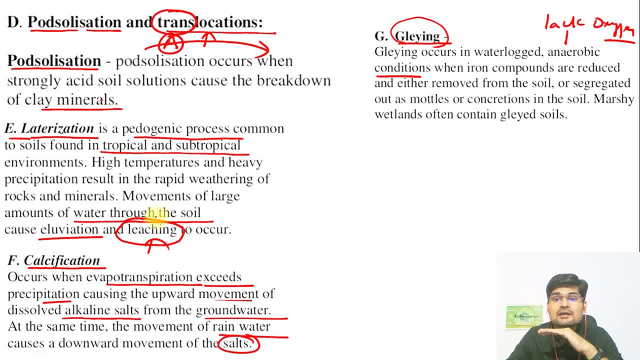 lack of oxygen. that is anaerobic condition where you have completely marshy or wet wetlands. when the iron compounds are reduced and either removed from the soil or segregated out as mortals or congregations right, That is important in the soil and generally the 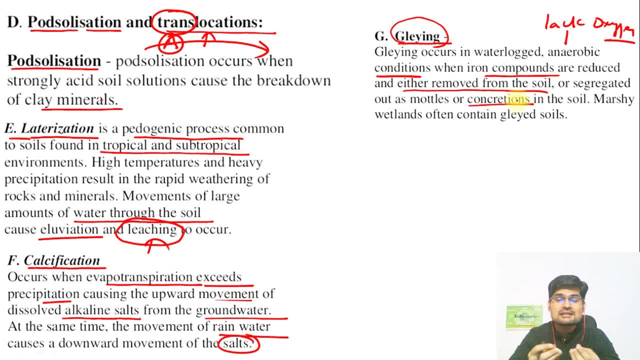 marshy or wetland areas where you have complete water coverage. there, when there is a decomposition in the soil under anaerobic process, that is the process where it is called glaying. So glaying is also one of the important processes and remember the anaerobic, the lack of oxygen. 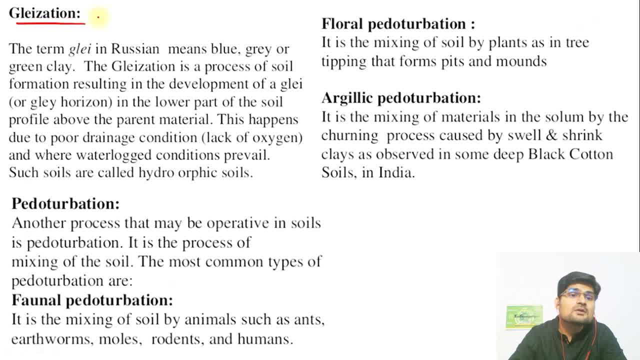 condition here. So glaying or glazation, Glazation is also the same word here, and the term glay is coming from the Russian word, which basically means blue, green or the clay right. So glaying or glazation is a process. 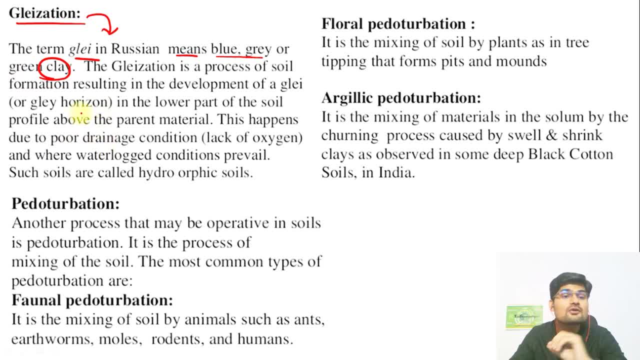 of soil formation, resulting in development of a layer or a horizon, called glay horizon, which is largely clay, like right, And this happens due to poor drainage condition, because it is waterlogged area, as we have learnt right. Apart from this, there is another process which is related to a word called turbation. 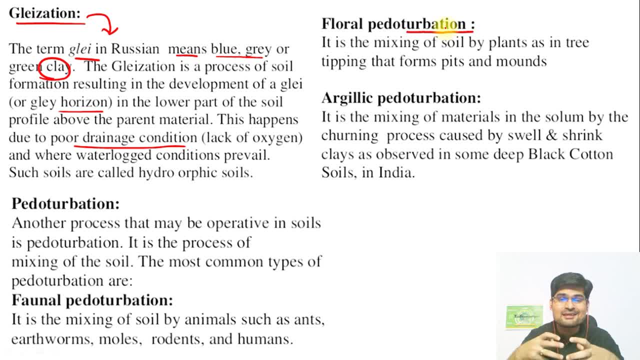 and remember, turbation is nothing but mixing of soil, right? So what happens? There is something called paedoturbation as a process that we must understand. Paedo is basically coming from soil, So when soil is mixed in different environment, it is called paedoturbation. 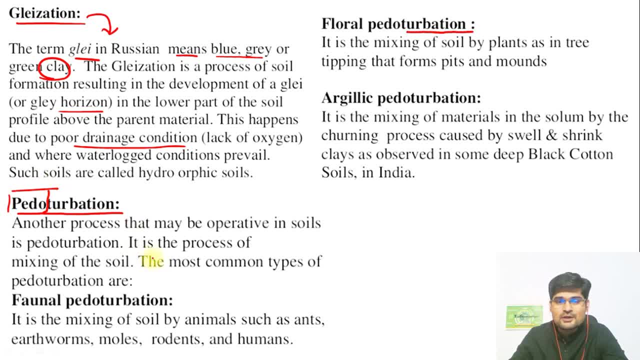 So it is another process that is important for the formation of soil. So it is the process of mixing of the soil, where the most common types of paedoturbation are faunal paedoturbation, floral paedoturbation and argillic paedoturbation. 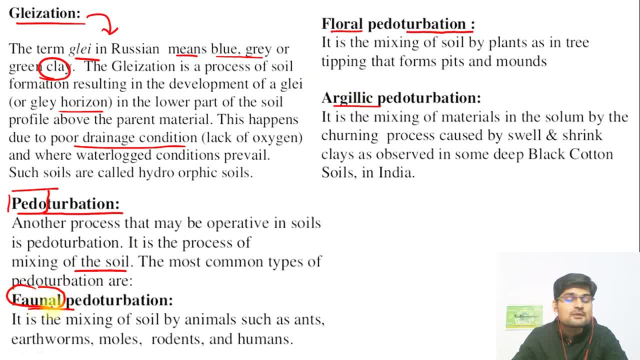 So the word itself is faunal. Fauna means coming from animalia kingdom, So animals such as ants, earthworm, moles, rodents, humans, right When these are decomposed and mixed in the soil horizon, that is called faunal pedoturbation. 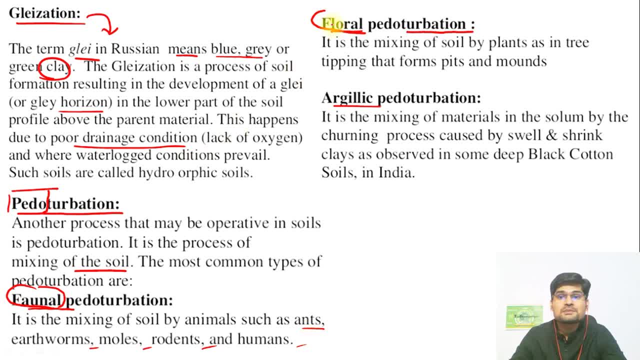 While, at the same time, if we have floral pedoturbation, it basically means soils are mixed with the plant remains right In the pits and mounds. that's important, And there is something called argillic pedoturbation as well. 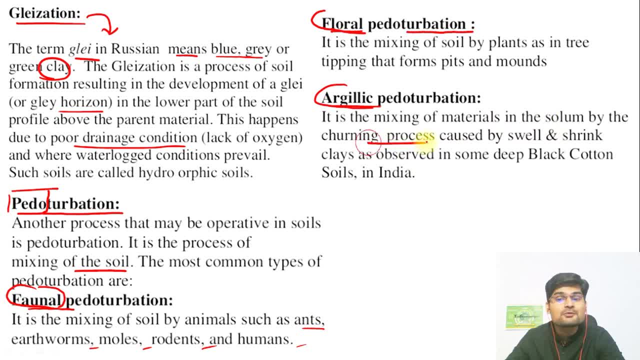 So it is mixing of materials in the soil by churning process. Remember the churning process, the movement caused by swell and shrinking clays, as observed in very deep black cotton soils, especially in India, if you observe right. So this kind of swelling and mixing of soil under too much of moisture, that is called argillic pedoturbation.